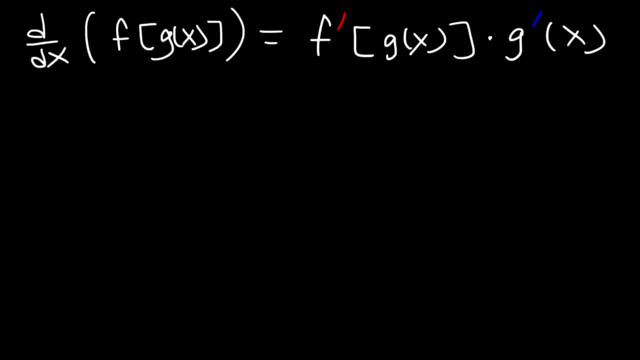 behind the chain rule. If you follow this process, you're going to get the answer right. So let's say, for example, if we have a function, u, raised to the n, where u is another function, in terms of x, Using the chain rule and the power rule combined, it's going to be n times u. 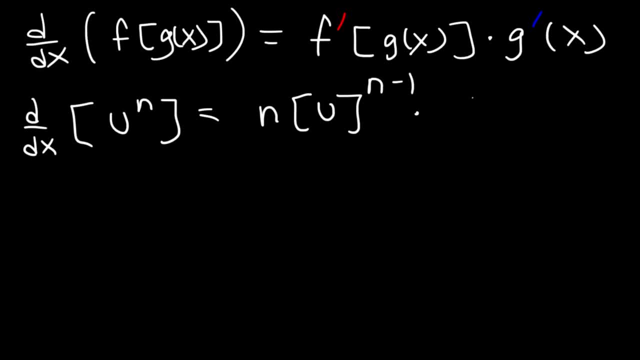 you have to keep that. the same, raised to the n minus 1 times the derivative of what's on the inside. That's the general power rule formula with the chain rule combined. So never forget to multiply by the derivative of the inside function. 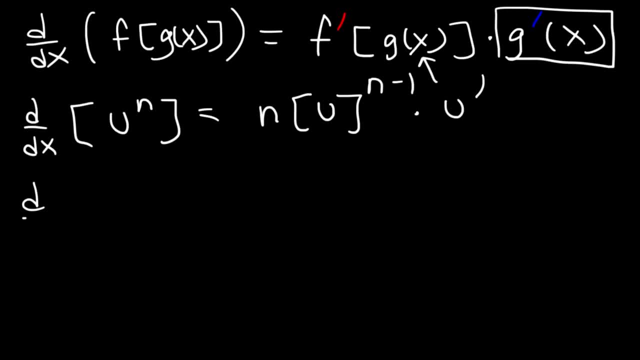 So let's use an example. Let's say, if we want to find the derivative of 5x plus 3, raised to the fourth power, So the first thing we're going to do is we're going to move the constant- I mean the exponent- to the front. 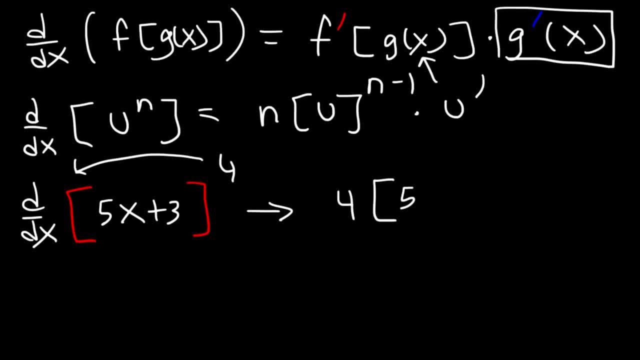 So it's going to be 4, and then keep the inside stuff the same times: 5x plus 3,. subtract the exponent by 1,. 4 minus 1 is 3, and then multiply by the derivative of the inside. 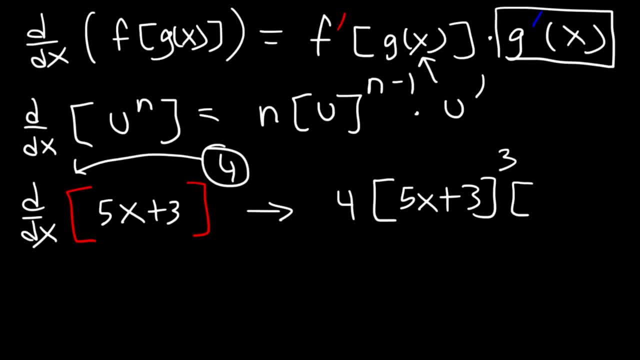 The inside function is 5x plus 3.. The derivative of 5x plus 3 is just 5.. So that's the answer. We can multiply 4 and 5, that's going to give us 20.. So it's 20 times. 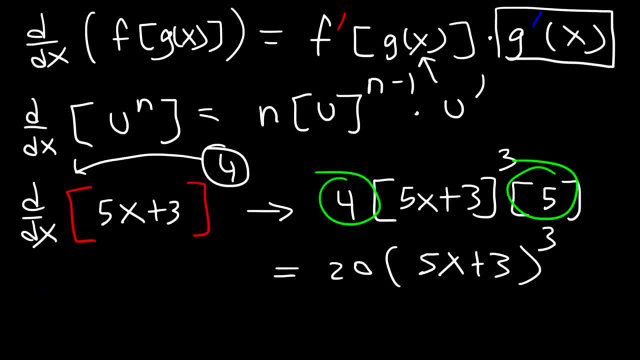 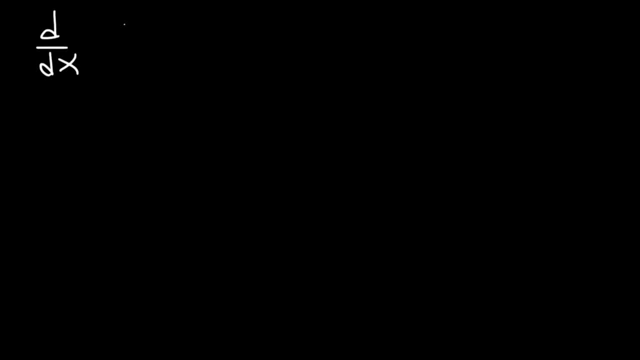 5x plus 3. 3 raised to the third power. So that's the final answer, fully simplified. Now let's work on some more examples. Find the derivative of x squared minus 3x raised to the fifth power. So first, 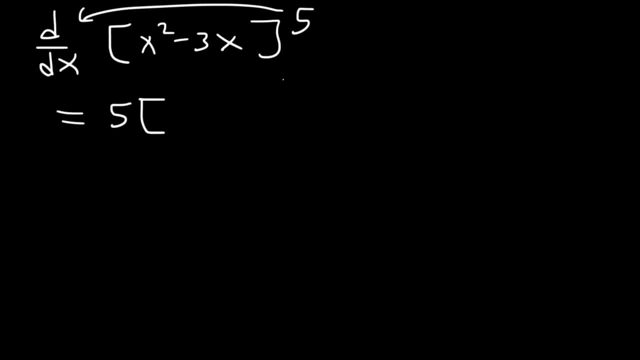 let's bring down the 5.. So it's going to be 5, and then keep the inside function the same and then subtract the exponent by 1, so this is 4, and then multiply it by the derivative of the inside. The derivative of x squared minus 3x is 2x minus 3, and so that's the answer Once you. 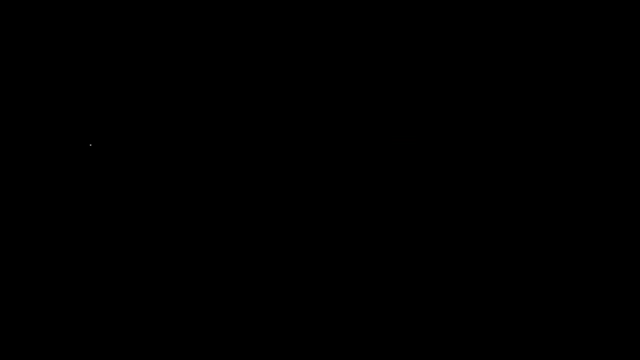 get used to the process, it's not that bad. Here's another example that you can try. Find the derivative of sine of 6x. The derivative of the outside part of the function sine is cosine and you got to keep the inside function the same. Then you multiply it by the derivative of the inside. 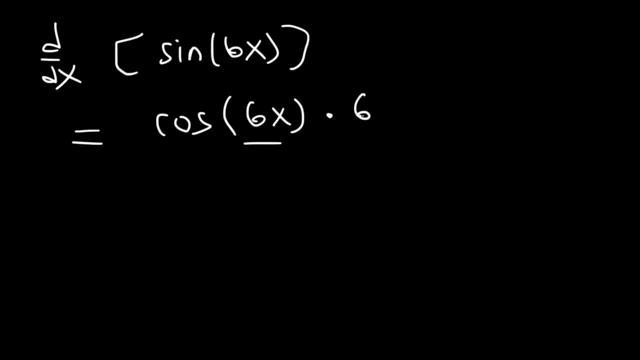 function. The derivative of 6x is 6, so the answer is simply 6 cosine 6x. Now what is the derivative of cosine x squared? So first differentiate the outside part of the function: cosine. The derivative of cosine is negative, sine. Now the inside part of the function. 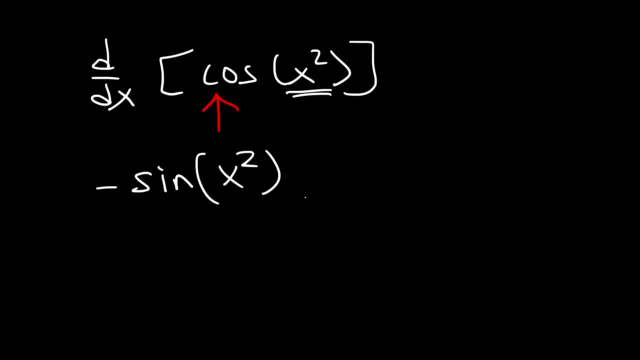 has to remain the same angle of cosine, so it's going to be x squared, And then differentiate the inside function x squared, which is 2x. So basically you're working away from the outside towards the inside. The final answer is negative: 2x sine x squared. 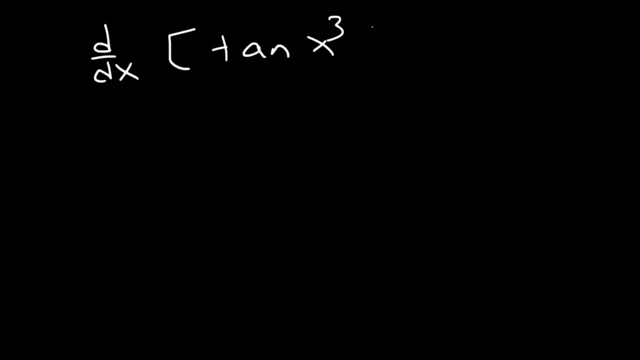 Find the derivative of tangent x cubed. So first let's differentiate tangent. The derivative of tangent is secant squared, and the inside function has to remain the same. Next, differentiate the inside function x cubed, So that's 3x squared and it's always multiplication. 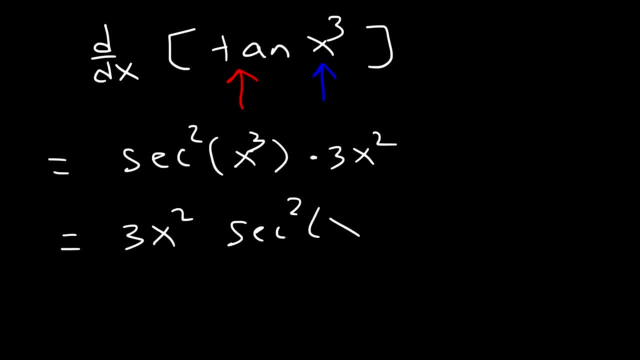 So it's going to be 3x squared- secant squared x cubed. As you can see, it's not that bad. Here's another problem: What is the derivative of secant 4x? The derivative of secant 4x is going to be secant tangent. 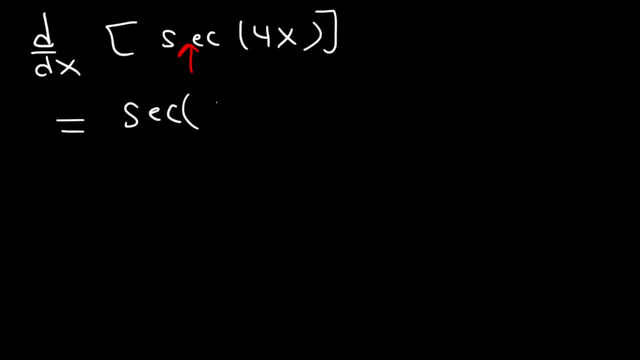 That's the derivative of secant. Now the inside function has to remain the same for secant and tangent. Next, we need to differentiate 4x, so it's just going to be times 4. And so that's the solution. 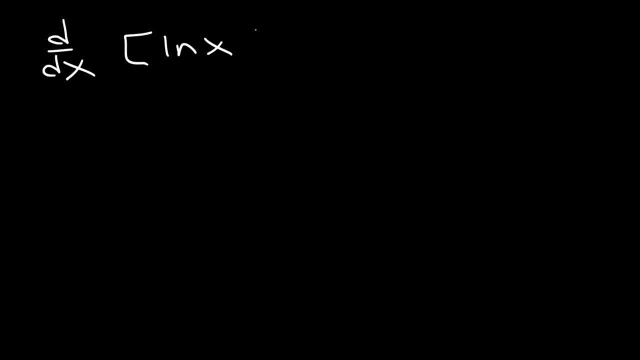 What is the derivative of ln x raised to the seventh power? Try that problem. Okay, Here's the problem. So this is going to be 7, keep the inside part the same and then subtract the exponent by 1.. So 7 minus 1 is 6.. 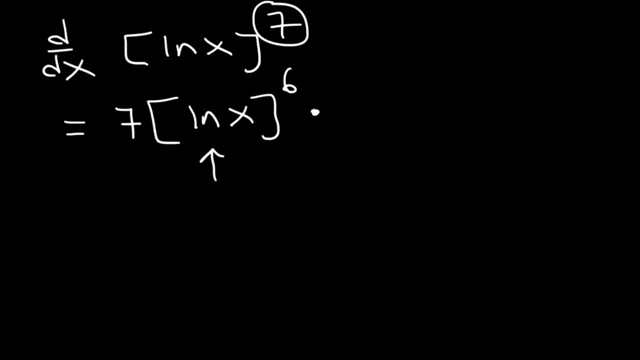 Now we've got to multiply by the derivative of the inside function. The derivative of ln x is simply 1 over x. So the final answer is 7 ln x raised to the sixth power, divided by x. The drug goes in this first set like so: 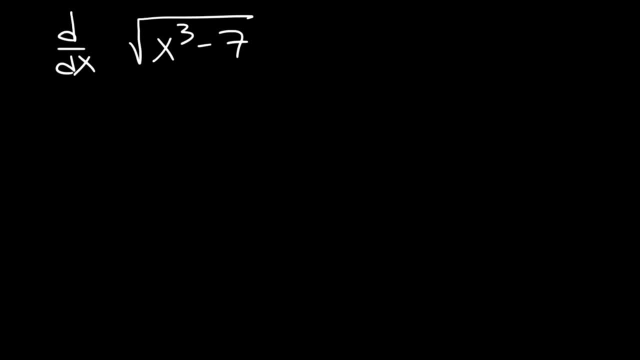 There it goes, So we're not going to get panic attacks, it's just going to be some 새로운 Wheels for today. Remember we discussed certain equations where you have to separate x from the substances that are going to silver. 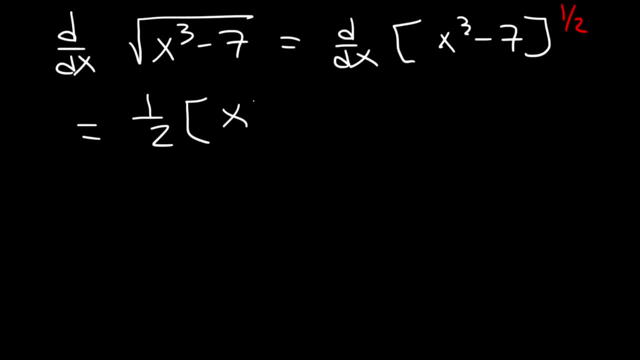 But there's no chance that it's going to work, So we're going to do this again. 削 outside oldest one by 1.. 1 half minus 1, which is 1 half minus 2 over 2, that's a negative half. And then we've got to. 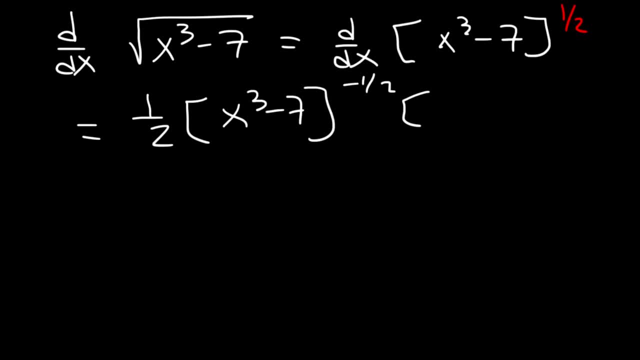 multiply by the derivative of the inside. The derivative of x cubed minus 7 is simply 3x squared, So we can bring this back to the bottom, since it has a negative exponent. So it's 3x squared divided by. we have a 2 on the bottom, 2x cubed minus 7, and now the exponent is: 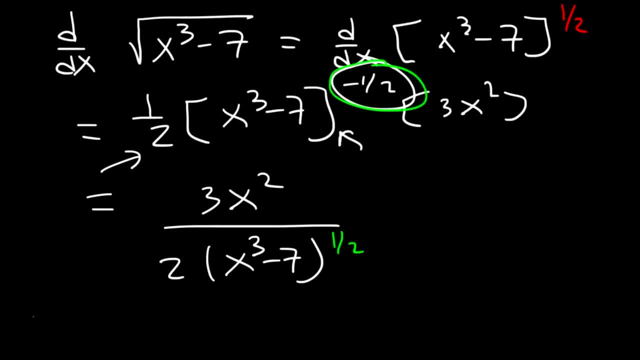 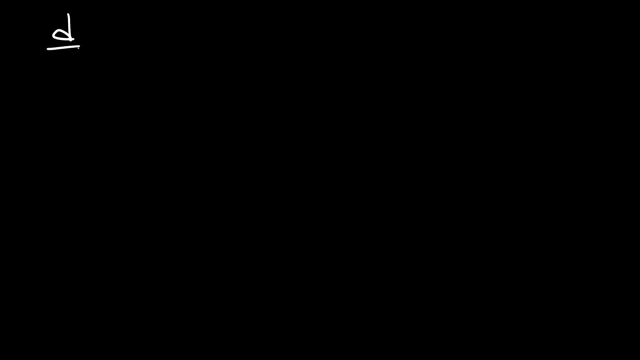 going to change from negative half to positive half, And now we can put it back in its radical form. So it's 3x squared divided by 2, square root, x cubed minus 7.. And so that's the final answer for this problem. Find the derivative of 1 divided by x squared, plus 8 raised to the third power. 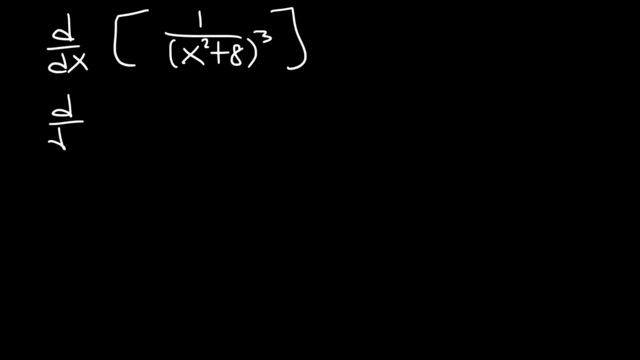 So first let's rewrite the expression. Let's bring the variables to the top. So this is x squared plus 8 raised to the minus 3.. And now we can use the chain rule combined with the power rule. Let's move the negative 3 to the front. 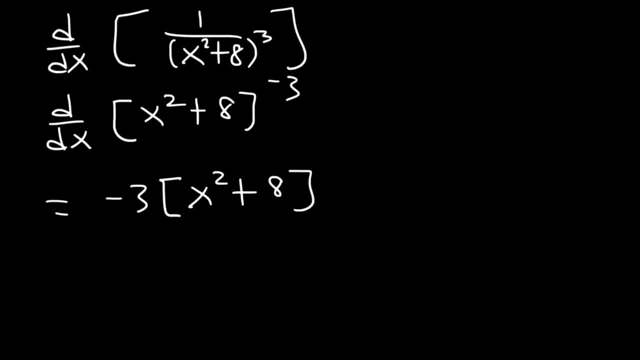 And let's keep the inside function. Let's rewrite it exactly the way we see it, And then let's subtract this by 1.. Negative 3 minus 1 is negative 4.. And now let's multiply by the derivative of the inside function, which is 2x. 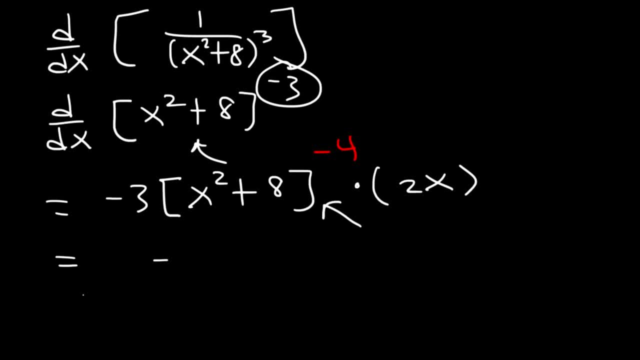 So now let's take this term and move it back to the bottom, So we have negative 3 times 2x, which is negative 6x on top, And on the bottom it's x squared plus 8 raised to the fourth power, And so that's all we need to do for this problem. 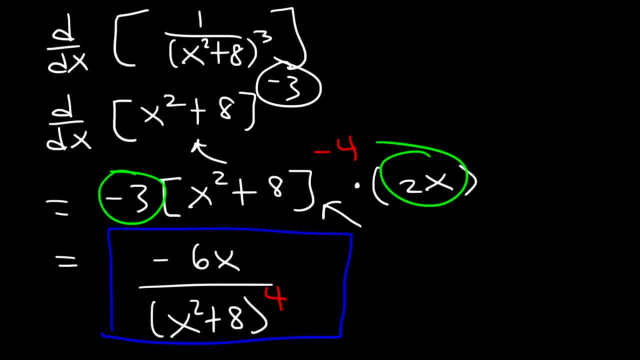 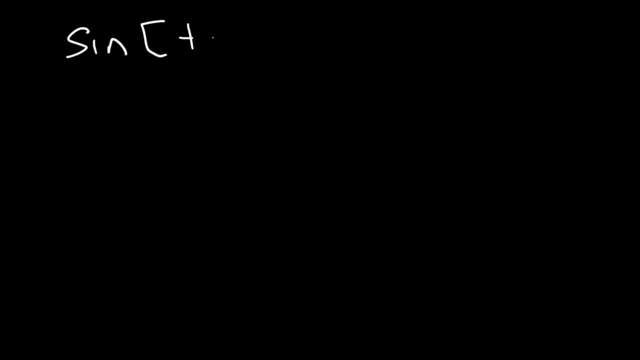 So for some examples you need to rewrite it before you find the derivative. Now what if we have a trig function inside another trig function? Find the derivative of this function. So first we need to differentiate the outside function, sine. The derivative of sine is cosine. Now what's inside of cosine, Since cosine came from sine? 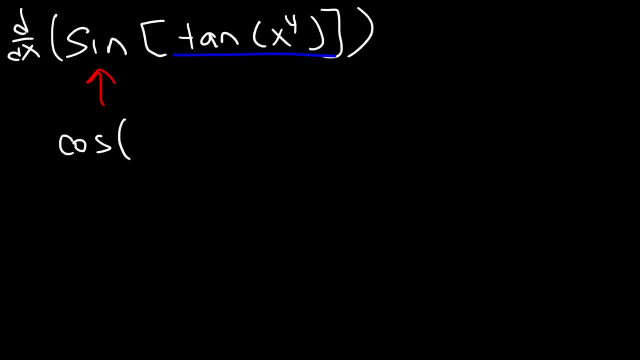 everything inside of sine is going to be the stuff inside of cosine. So that's tangent x to the fourth. Now let's move on to tangent. The derivative of tangent is secant squared, And the stuff that's inside of tangent is going to be the stuff that's inside of secant squared. 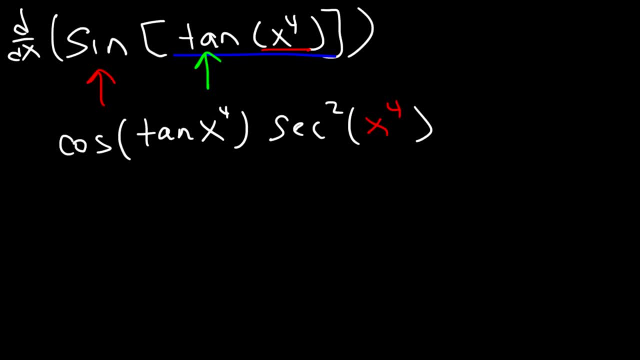 So that's x to the fourth, And then we've got to move on further towards the inside. The derivative of x to the fourth is 4x cubed, And so that's the answer. How about this example? Find the derivative of sine raised to the fifth power tangent. 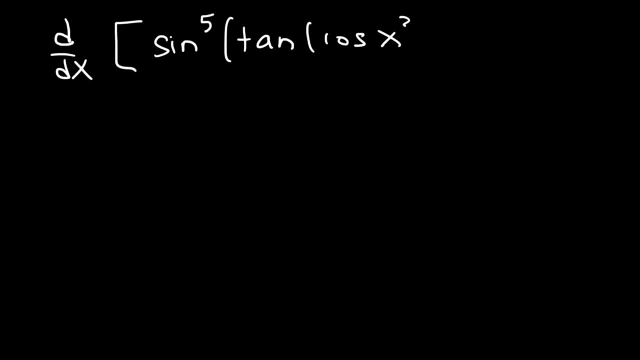 cosine x, cubed. The first thing I would do is rewrite the expression. So this is sine tangent: cosine x, cubed, all raised to the fifth power. So first let's deal with the exponents, Let's use the power rule. 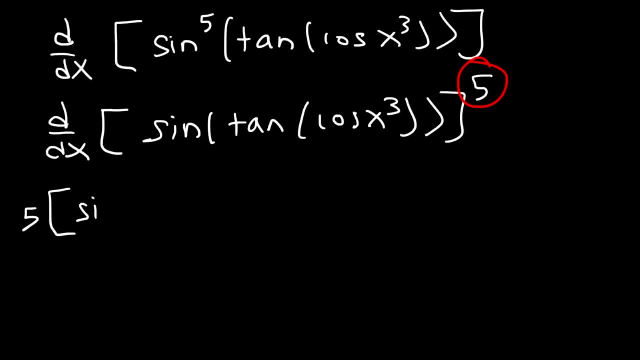 So we've got to bring the 5 to the front and keep everything inside the same. So always start with the outside portion, Which is going to be the exponents in this case, And then subtract the exponent by 1, so it's going to be 4.. 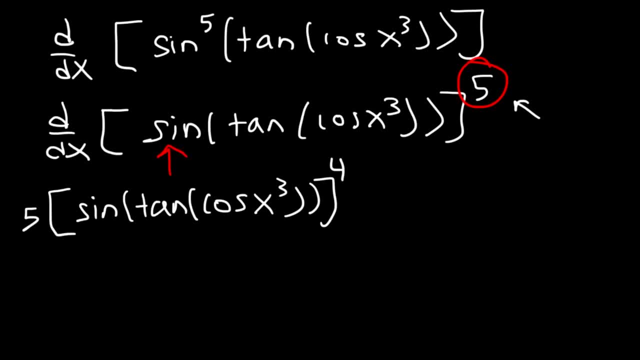 Now let's work our way towards the inside. So we've got to differentiate sine- The derivative of sine is cosine, And the stuff inside of sine is tan cosine x cubed. So we've got to put that here. Now let's move on to tangent. 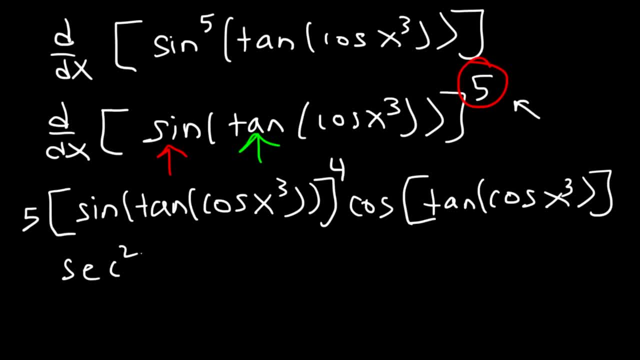 The derivative of tangent is secant squared, And the stuff inside of tan is cosine x cubed. So hopefully you're seeing a pattern with the way we're finding the derivative of everything. So now that we're done with tangent, let's move on to cosine. 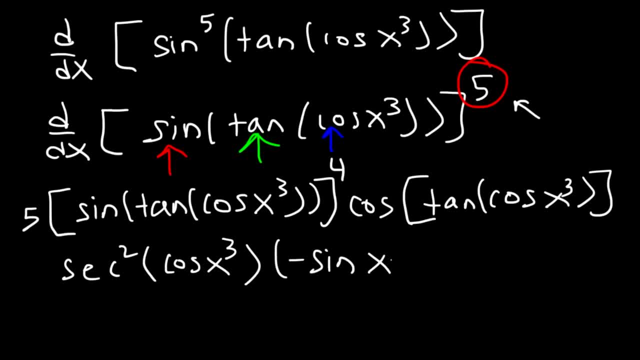 The derivative of cosine is negative sine And the angle of cosine is x cubed. so that's going to be the same here. And then let's move on to x cubed. The derivative of x cubed is 3x squared. 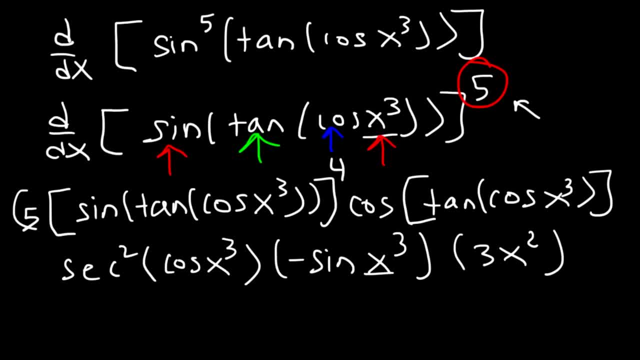 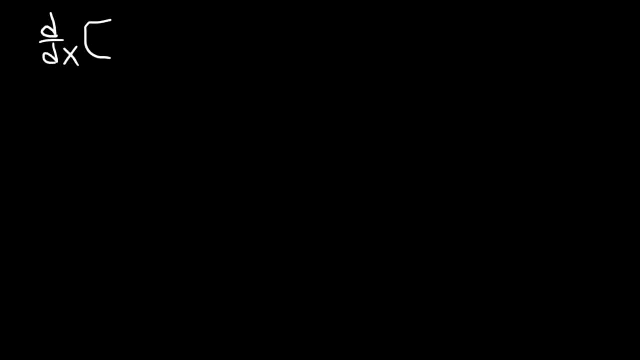 So that's the answer. and then you can combine terms, you can multiply 5 and 3 to get 15. what is the derivative of cosine raised to the seventh power of sine of secant x squared? so try that problem. so first let's rewrite it as cosine of sine of. 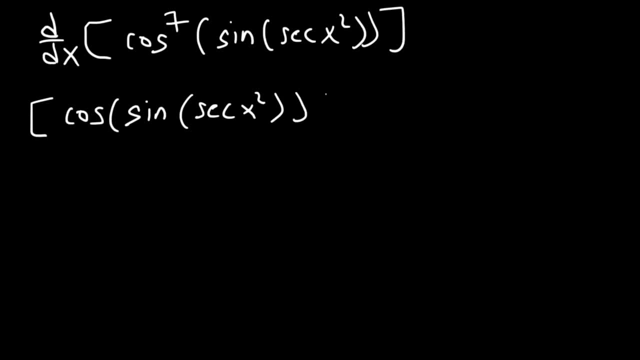 secant x squared. now let's put the 7 and its exponent position. so let's use the power rule, let's bring the 7 to the front and let's keep everything on the inside the same, and then subtract the exponent by 1, so this is going to be 6. 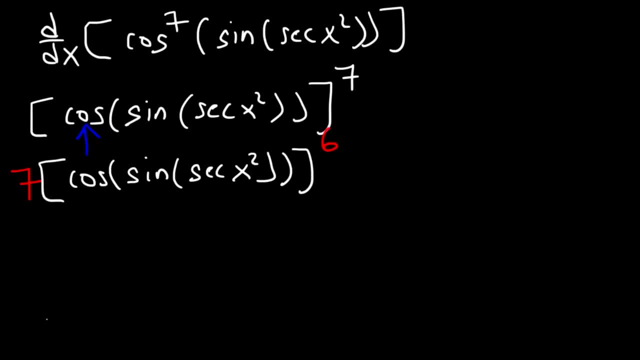 now let's find the derivative of cosine. let's work our way towards the inside. the derivative of cosine is negative sine and the stuff inside of that is sine, secant x squared. so now we got to find the derivative of sine. the derivative of sine is cosine and the stuff inside of sine is secant x squared. 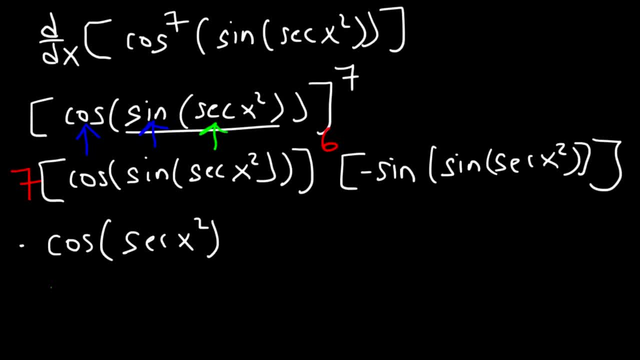 so now we got to find the derivative of secant, so that's secant, tangent. so it's gonna be secant x squared, tangent x squared, and the derivative of x squared is 2x. so whenever you have multiple composite functions, just work your way from the outside towards the 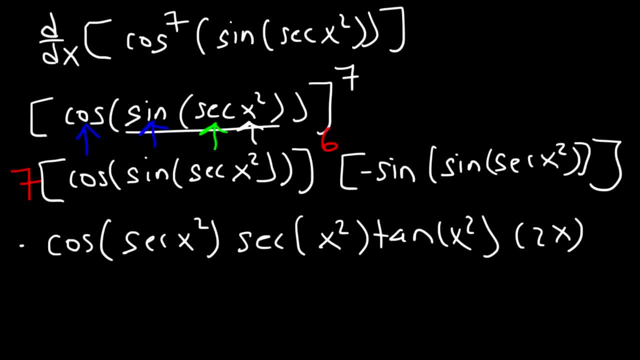 inside and everything is multiplied by each other and then, when you're done, simply collect terms. so we have a 7, a 2x and a negative. so you can move that to the front and write it as a negative 14x if you want to. here's the next problem. 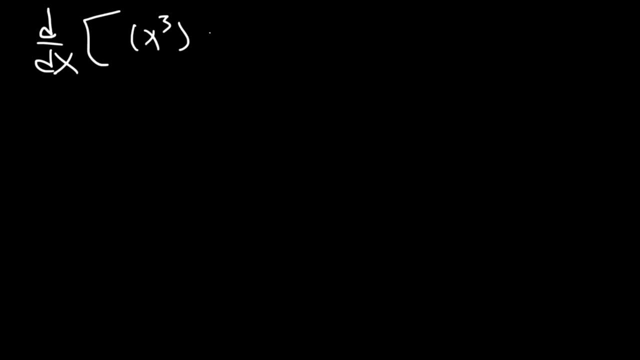 find the derivative of x cubed times 4x plus 5 raised to the fourth power. so what we have here is a product rule. we could say that this is F and this is G, and for G we have to use the quotient rule. I mean, that's the quotient, but the 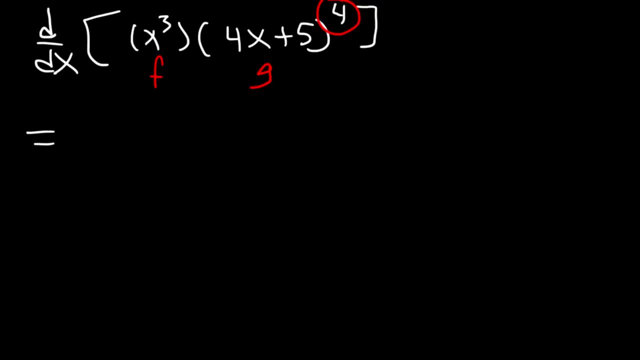 chain. so, using the product rule, we need to differentiate the first part F. the derivative of the first part is 3x squared and we need to keep the second part the same. So we just have to rewrite g Plus now. we need to keep the first part the same. 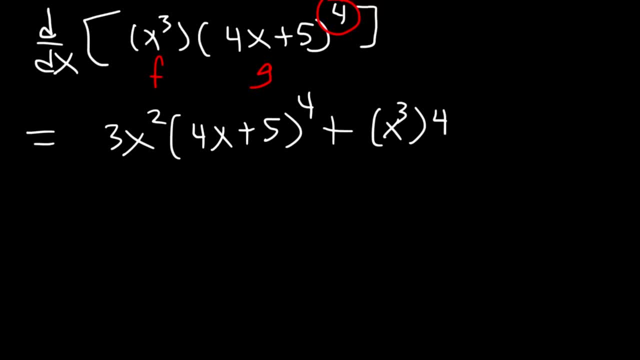 Now for the second part. we need to use the chain rule. So let's bring the 4 to the front, let's keep the inside stuff the same and subtract the 4 by 1, then multiply it by the derivative of the inside function. 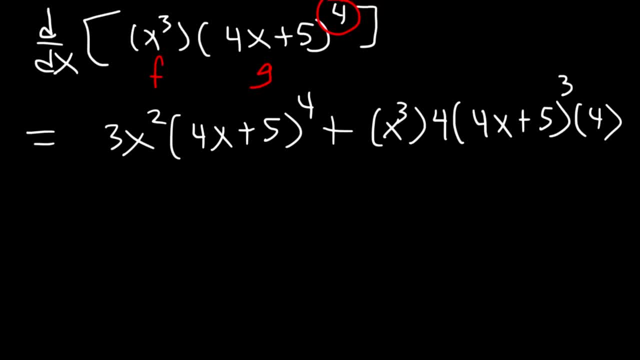 which is 4x plus 5.. The derivative of that is 4.. So now let's simplify. So the first part, we don't really need to change anything, We can just leave it like this. Now for the second part. we can multiply 4 and 4.. 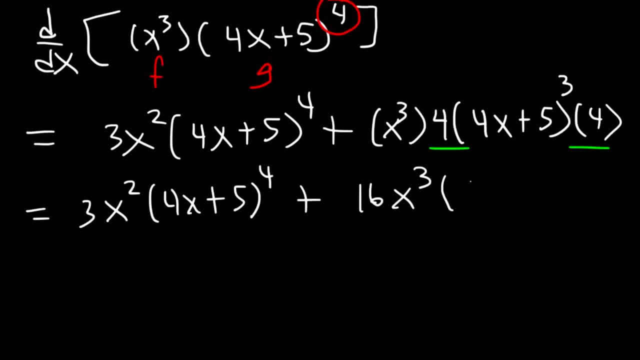 That's 16.. So this is 16x cubed times 4x plus 5, raised to the third power. You can leave your answer like this or, if you want to, you can take out the GCF. We can take out an x squared. 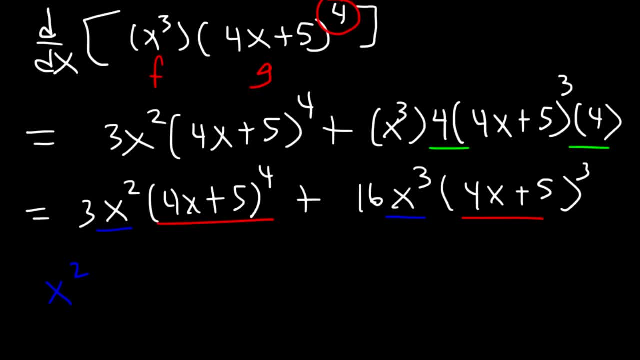 and we can take out 3, 4x plus 5s, or basically 4x plus 5 to the third power. So this is gone and we took 3 of these. One is left over and we have a 3 left. 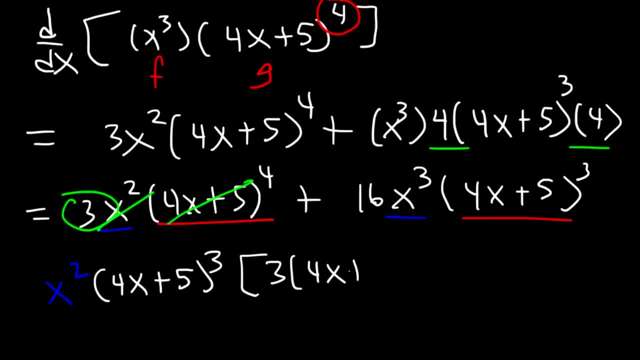 So this is going to be a 3 times 4x plus 5, and this is gone. We took out all 3 of these. Well, there's an x left over and it's 16,, so plus 16x, because we took out an x squared. 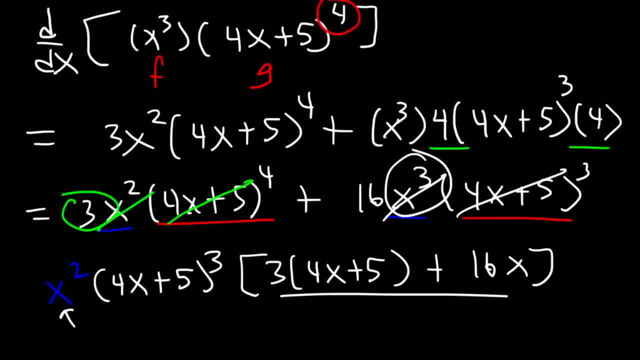 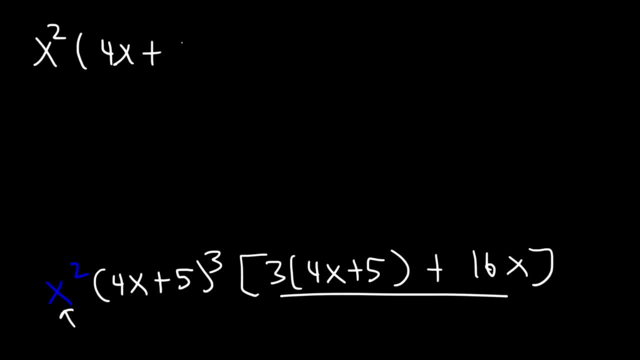 Now what we can do is basically simplify what we have here. So this is x squared 4x plus 5 to the third power and let's distribute the 3.. So 3 times 4x is 12x, 3 times 5 is 15, plus 16x. 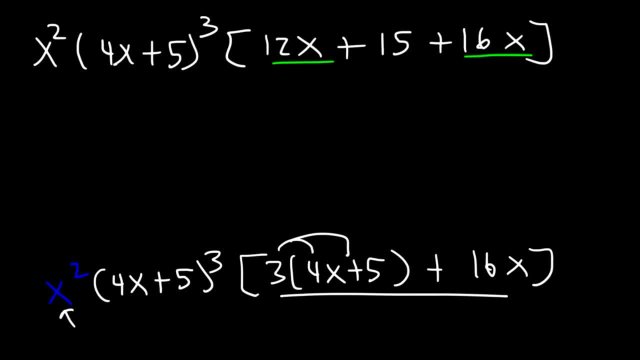 Now let's add 12x and 16x, So the final answer is x squared times 4x plus 5 to the third power, and then 28x plus 15.. So that's the solution. Let's try one more example. 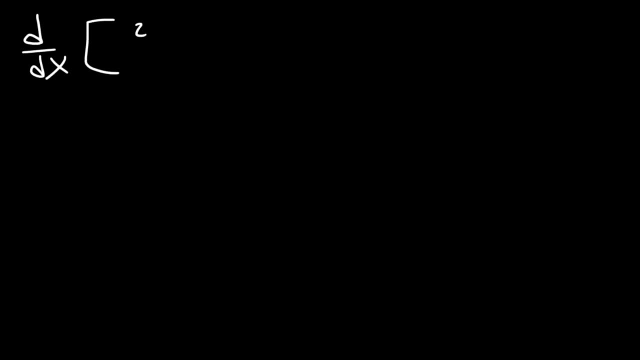 Let's find the derivative of 2x minus 3 divided by 4 plus 5x, raised to the fourth power. So this is a chain rule and quotient rule problem. So first we need to bring the exponent down and keep the stuff on the inside the same. 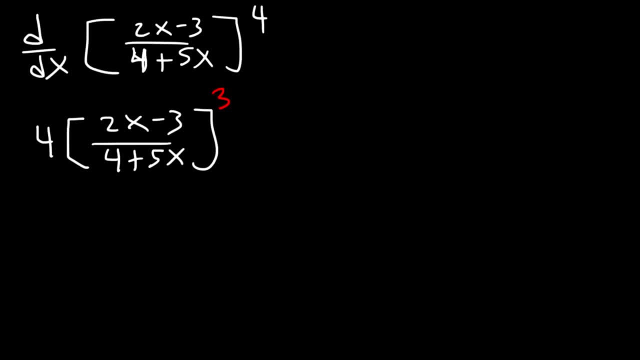 and then subtract the exponent by 1.. Next, we'll need to multiply by the derivative of the inside, So that's when we have to use a quotient rule. So f is 2x minus 3, and g is 4 plus 5x. 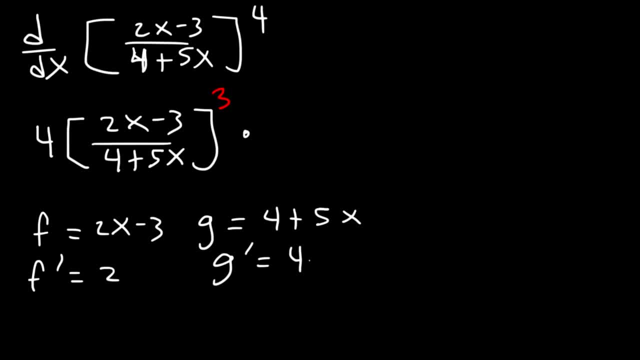 f prime is 2, g prime is 4.. And the formula for the quotient rule is: it's gf prime minus fg prime over g squared. So g is 4 plus 5x, f prime is 2, and f is 2x minus 3.. 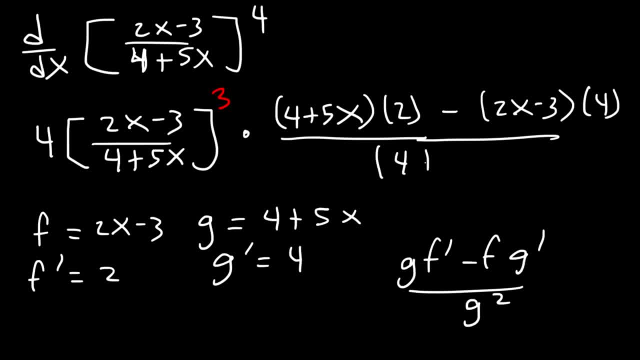 g prime is 4 divided by g squared, which is 4 plus 5x squared. So, as you can see, this is a long problem. So let's simplify what we have on the right side. If we distribute the 2, it's going to be 8 plus 10x. 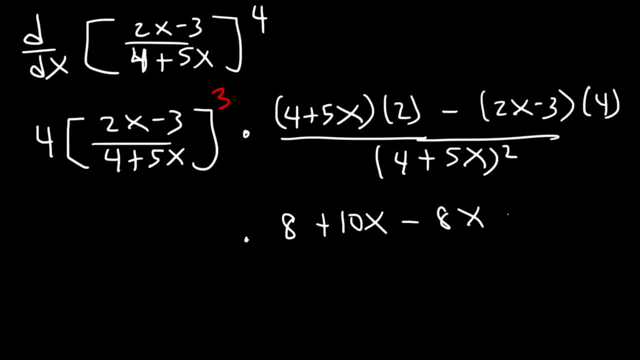 And if we distribute the 4, it's going to be negative 8x, And then negative times negative 3 times 4, that's positive 12.. Divided by 4 plus 5x squared, And then this part is going to be the same. 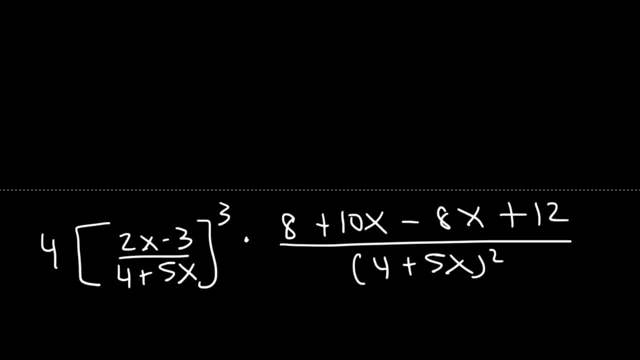 So let's simplify the numerator. So first we can add 8 and 12. So that's going to be 20. And then 10x minus 8x, that's positive. 2x Divided by 4 plus 5x squared.